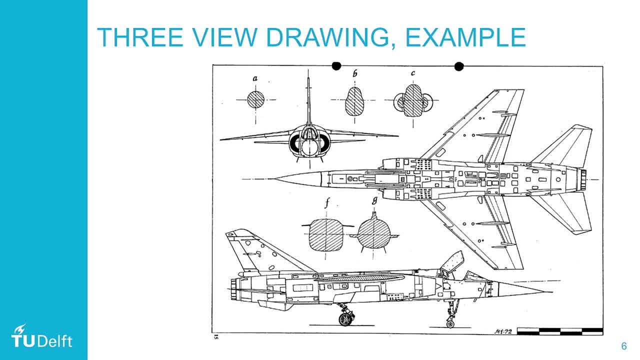 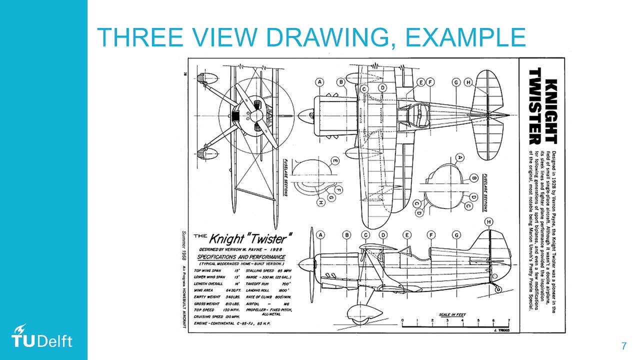 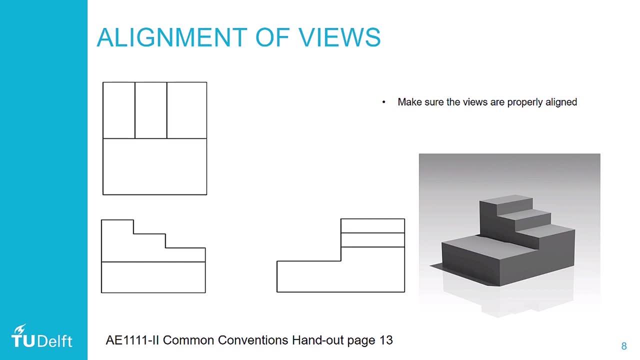 are given to provide a little more information on the geometry, And in this example you can see that the views are nicely aligned. This is very important for this assignment. During engineering drawing, you have learned that projection views should always be properly aligned. You can make use of this alignment to construct your geometry. You can transfer. 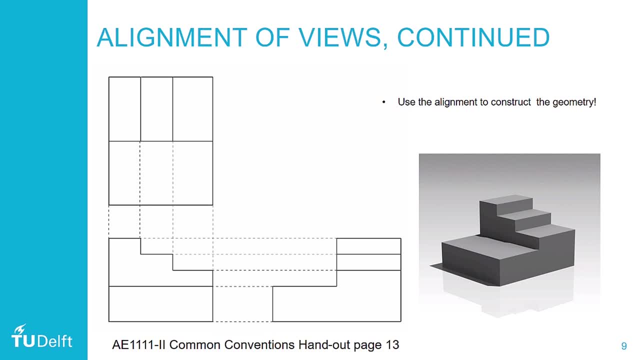 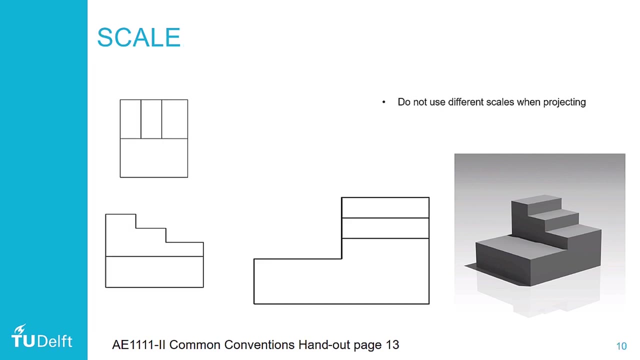 elements from one view to the other view using your ruler, So always properly align your items. Something which is visible from the top, inside and front should be present in each view. For the same reason, it is important to use the same skill when you project your. 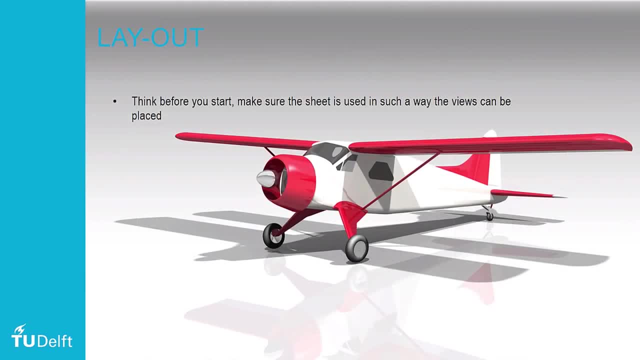 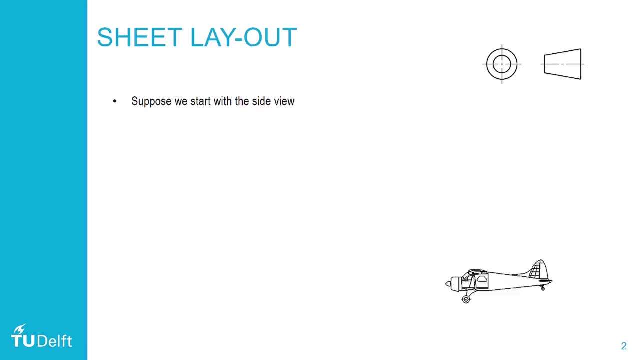 views. Please think before you start drawing your first view. Make sure that you use the sheet in such a way that all the views can be placed. Suppose you start with the side view. Relative to the side view, the top view can be placed. 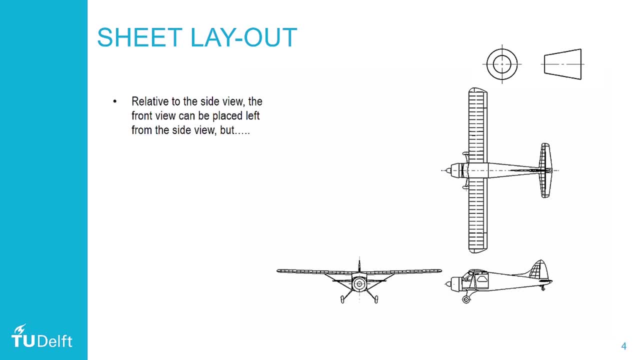 above it. Relative to the side view, the front view can be placed on the left, But the sheet might end up being too small to place this configuration. All views should fit on the sheet. The front view also can be positioned left from the top view. 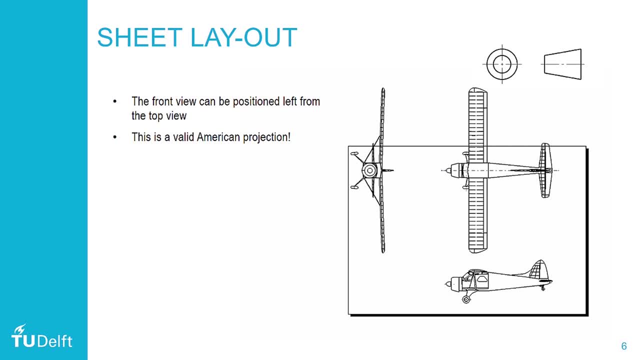 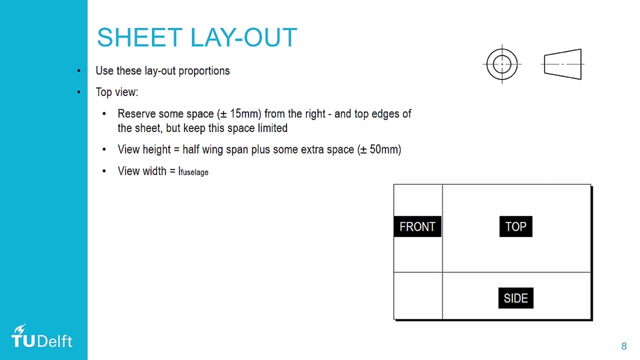 This is a valid American projection For this assignment. this is the proper layout of the views. You can leave out a single wing due to symmetry, but please draw the complete fuselage. So please use these layout proportions for this assignment. For the top view, reserve some space from the right and top edges for about 50mm. but 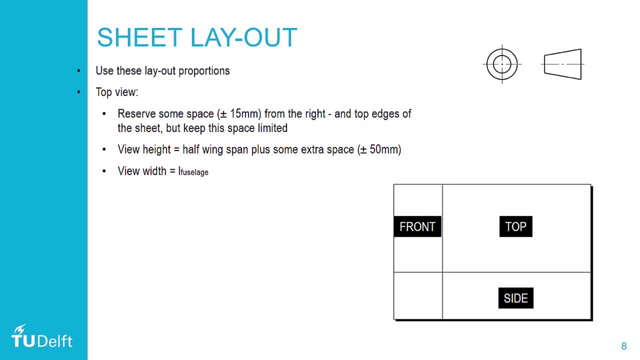 keep the space limited. The view height will be half the wingspan plus some extra space, coarsely 50mm. The view width is determined by the length of the fuselage. For the side view you should align it with the top view, so the view width is identical to the top view. The view height. 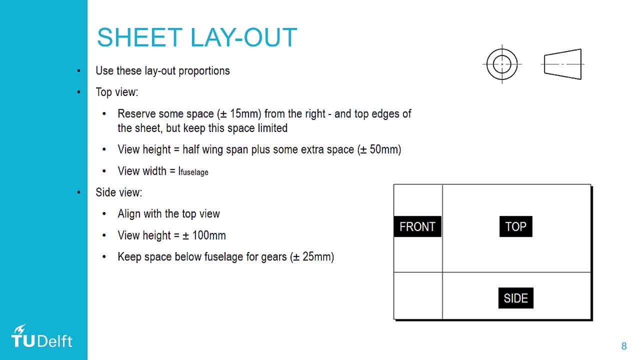 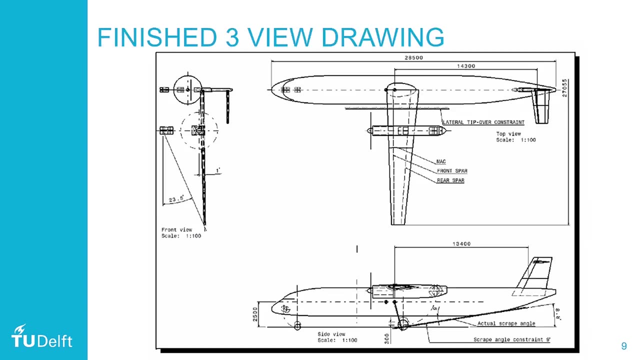 is about 100mm And make sure to keep some space below the fuselage for the gears, approximately 25mm. The front view can be kept about 50mm away from the left edge of the sheet. It should be aligned with the top view so that determines the position in the vertical direction.